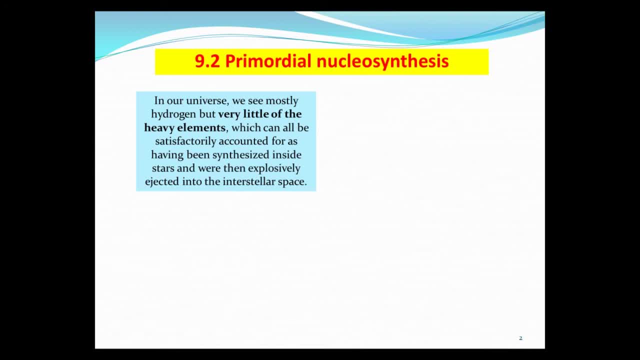 account for us, having been synthesized inside the star or then explosively ejected into the interstellar space. On the other hand, everywhere we look, besides hydrogen, we also see a significant amount of helium. The helium abundance can be deduced from the measurements. 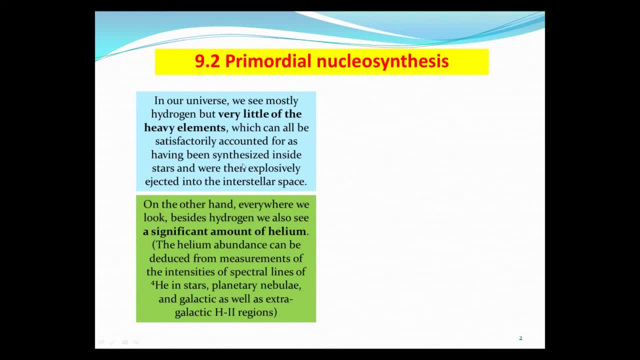 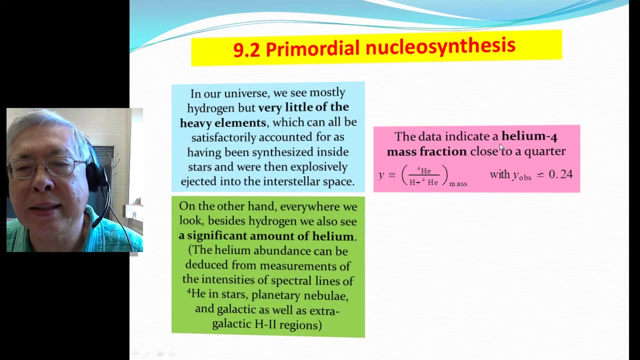 of intensity of the spectralized helium, for in the stars and planetary nebulas and galactic squares The data indicates helium for the mass fraction close to a quarter, which means all the mass is basically hydrogen plus helium divided by the mass ratio, which we'll call y. 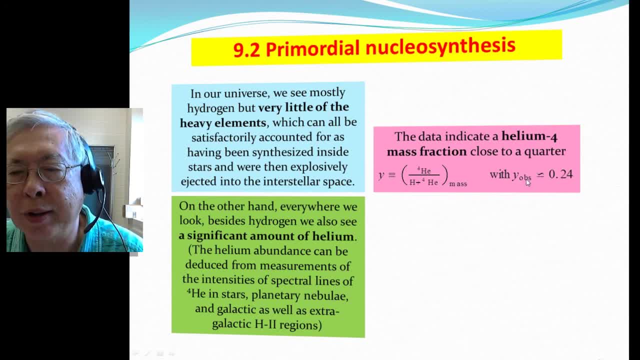 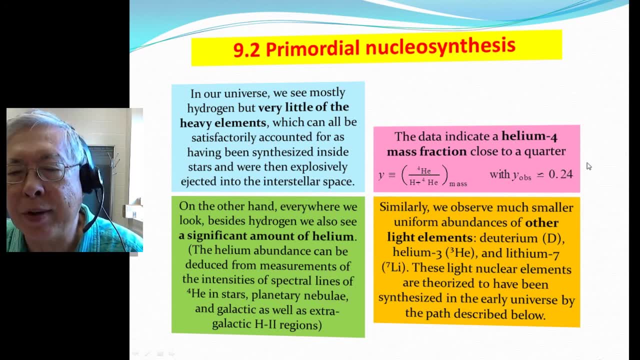 Similarly, we can observe much smaller uniform abundance of other light elements: deuterium, which is the isotope of hydrogen, with an extra neutron, helium-3, and lithium-7.. These light nuclear elements are theorized to have been synthesized in the early universe. However, 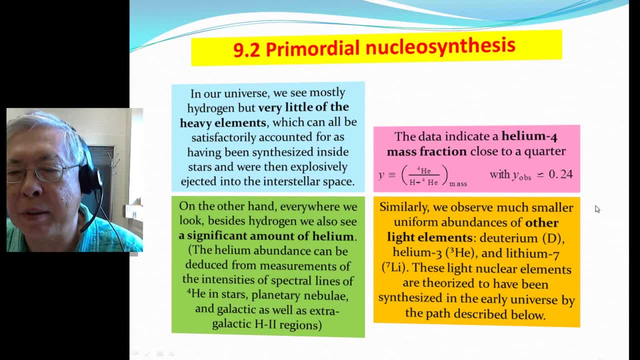 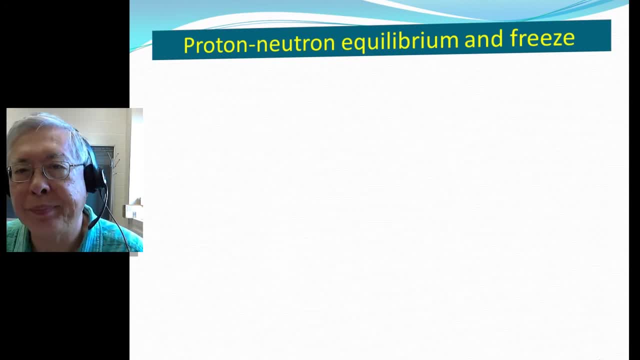 they are not known by the path we're going to describe. So these are the big band nuclear synthesis or the primordial nuclear synthesis we're talking about. First we'll talk about the epoch called proton-neutron equilibrium, or freeze out. 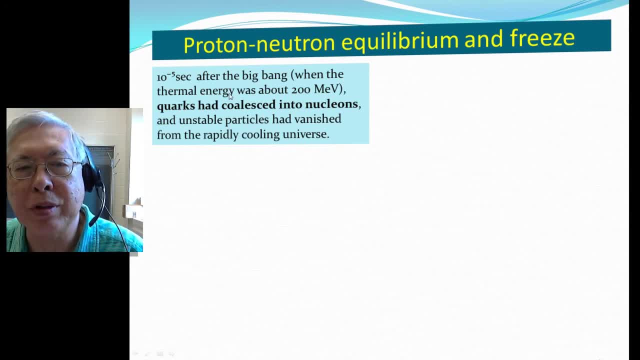 About 10 microseconds after the big band, when the thermal energy was about 200 MeV, quarks have coalesced into nucleons and the unstable particles have vanished from rapid cooling of the universe. The cosmic soup was then composed of protons, neutrons, electrons, positrons, three-flavored. 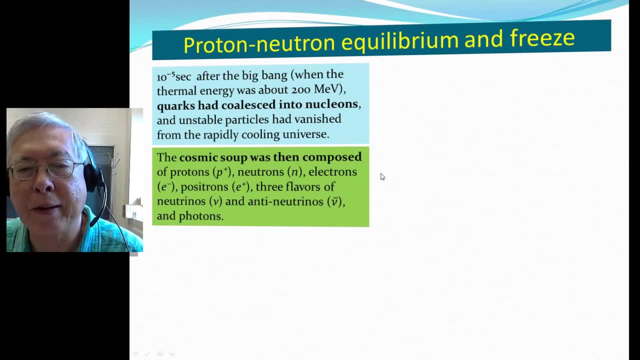 neutrinos and anti-neutrinos and photons. Sometimes we call this the era of nucleons. Up until the first second after the big band, Neutron-proton could interconverge with each other by weak interactions. For example, neutrons taking a positron can convert a proton plus an anti-neutrino or 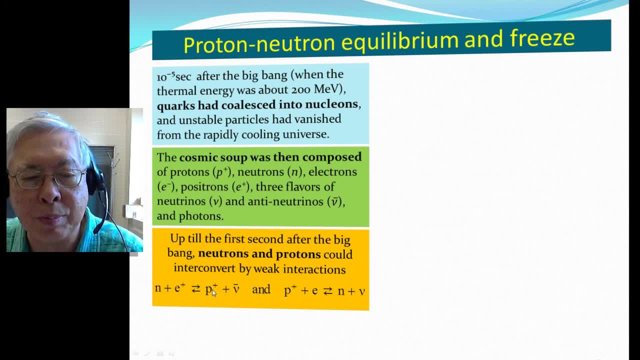 backwards anti-neutrinos. adding an inter-interacting with a proton can produce a neutron and a positron. same way, this reaction also. So neutron-protons are also about the same. So neutrons-protons are also about the same. 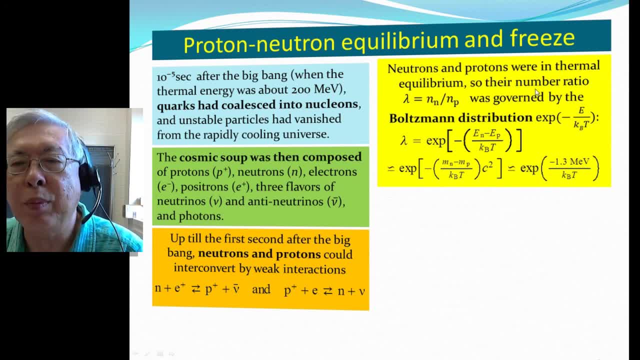 So neutrons-protons are also about the same, are in thermal equilibrium. So the number ratios, the number of neutrons divided by the number of protons called lambda, is governed by the Boltzmann distribution. See, the number is proportion x, e to the minus energy. 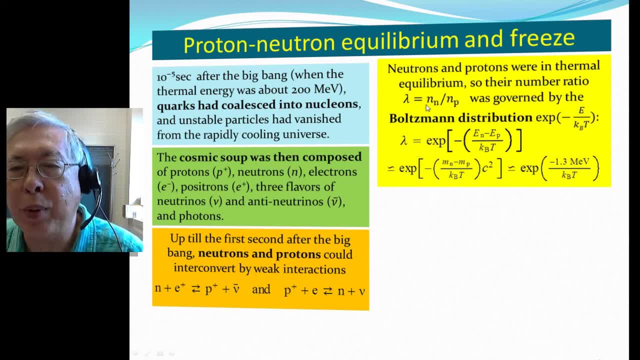 divided by kt And so therefore the ratio neutron and proton will be e to the minus electron energy, minus neutron energy, minus proton energy over kt, And the energy mostly is rest energy. So the neutron energy will be just the rest energy, neutron mc squared. 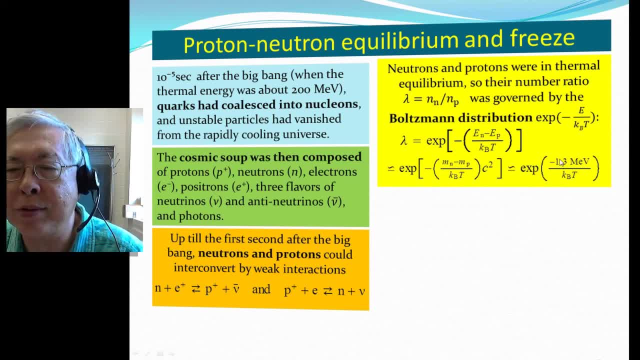 And here you just plug in the neutron-proton mass difference: 1.3 MeV. Neutron is slightly heavier than proton And you get this. So the number ratio should be in thermal equilibrium should be given by this. if you know the kt. 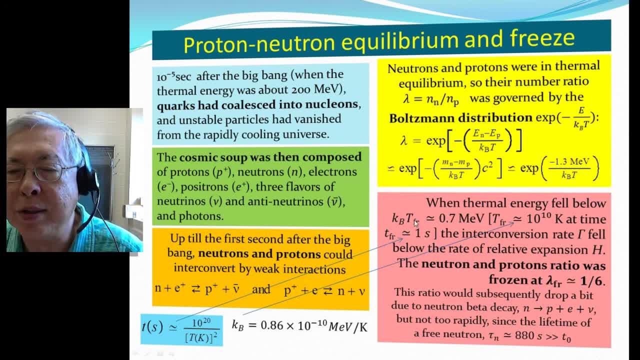 When the thermal energy fell below so-called the freezing point, which is about 0.7 MeV. MeV, you know, convert into temperature-wise. just divide by this, Divide by Boltzmann constant, you get about 10 billion kelvin. 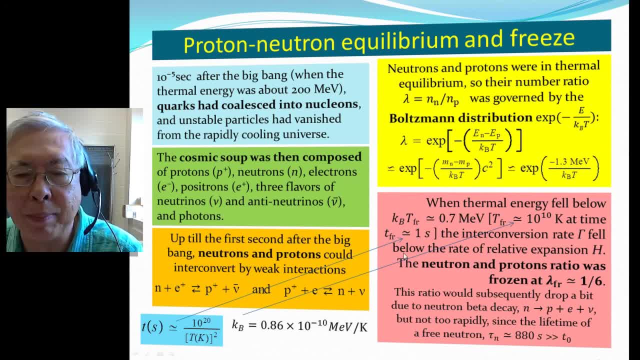 And this is about one second after the Big Bang, because, knowing the temperature, you plug in this formula, you get the cost of time in terms of seconds. about one second. Now. the interconversion rate gamma fell below the expansion rate h. 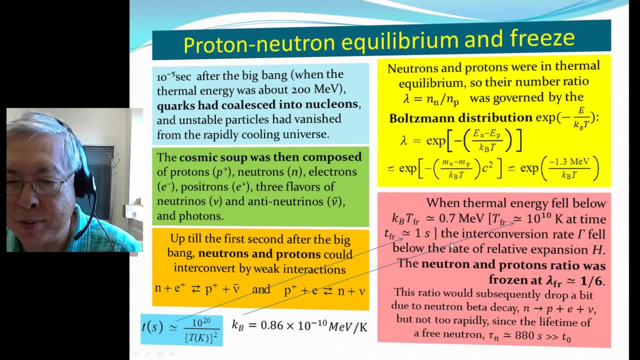 So that's how people arrived at 0.7 MeV. Now, once you know the fact that this is kt is 0.7 MeV, so divide that to 1.3 MeV and it will work out to be 1 over 6.. 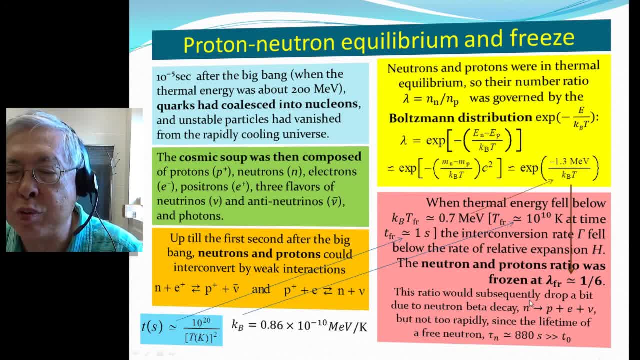 OK, And this number was set OK, So it's going to drop a little bit due to the neutron beta decay. Free neutron can decay into proton plus electron neutrinos, but not too rapidly, since the lifetime of free neutron is 880 seconds, which is of course. 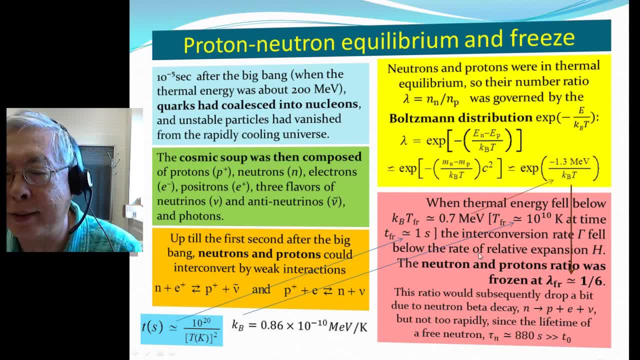 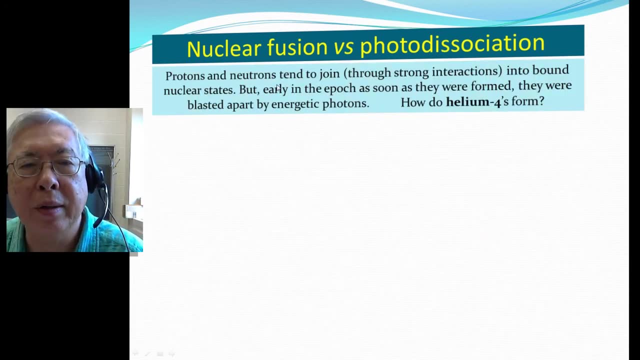 much bigger than the age of the universe, then about a few seconds. So it's only dropped a little bit. So now we can talk about the fusion of neutron proton into bound nuclear states, But early epoch, as soon as they were formed, for example. 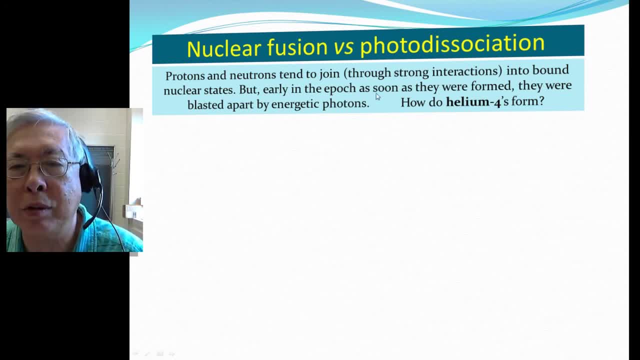 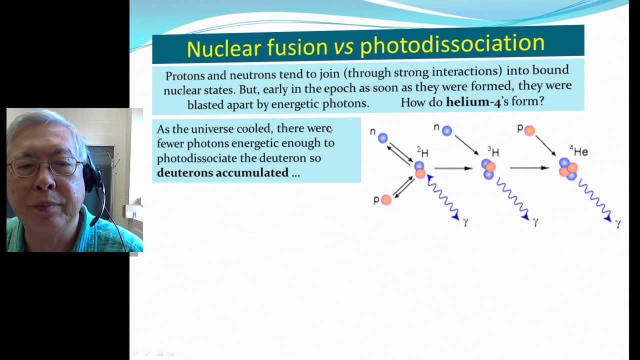 they were immediately blasted apart by energetic photon. so the photon dissociation. So the question: how do helium form formed? So the idea is a proton neutron. fusion of proton and proton fuse into a deuterium, which is said isotope of hydrogen, and produce a photon. 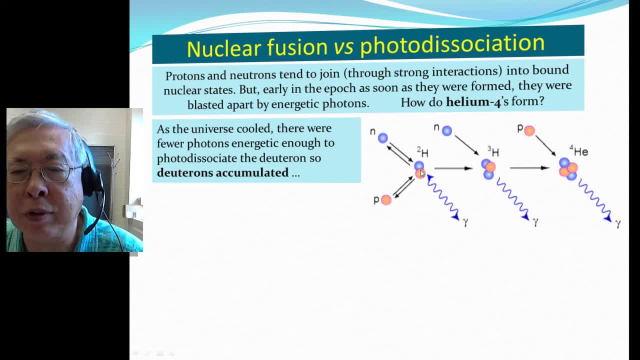 or can reverse. an energy, photon can further dissociate this deuterium and go back to neutron, proton. so all these reversible processes until the universe cool such way that the photons, the ambient photons, is not energetic enough to trigger the reverse reaction. so therefore proton, neutron turns into 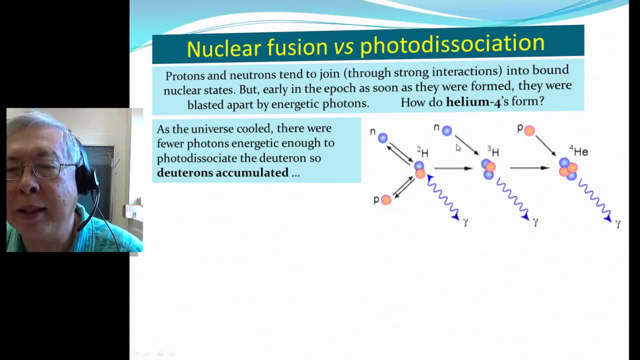 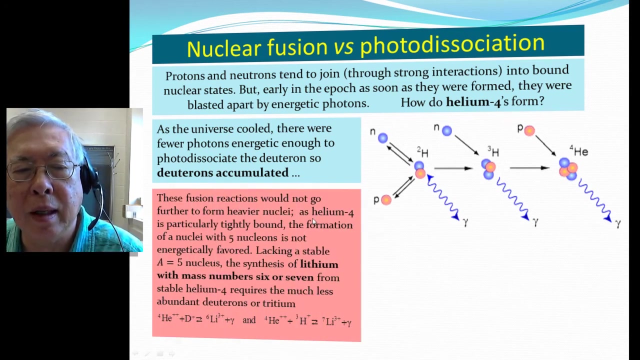 deuterium, and the deuterium combines another neutron emitting photon to become a tritium, the isotope of hydrogen, with two neutrons, and then combines another proton to form helium-4. and these fusion reactions will not go further to form heavier nuclear as. 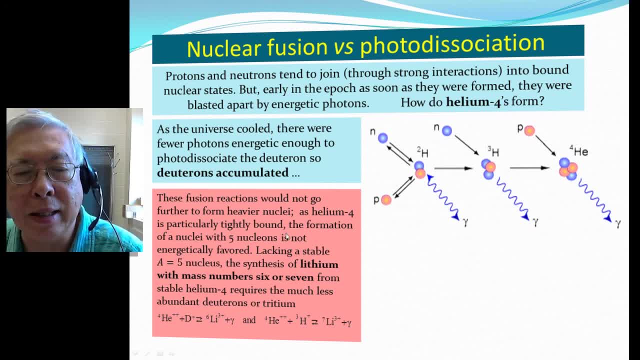 helium-4 is a particularly tightly bound state and the formation of nuclear with five nucleons is not energetic favored for the lacking of a stable mass five nucleus. the synthesis of lithium with mass number six- seven from stable helium requires a much less abundant deuterium and a much more stable helium with mass number six- seven from stable helium requires a much less abundant. 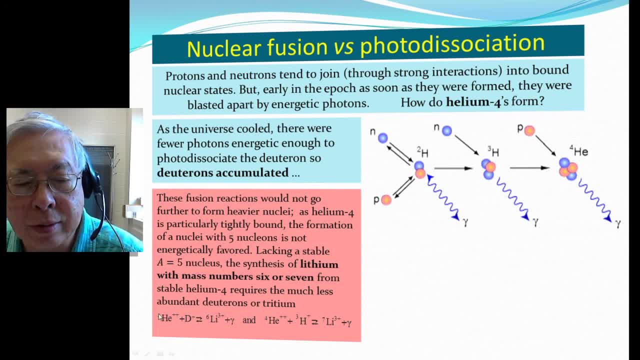 deuterium. you see, you had to find the human flight to find children, to make any lithium's or to fight Tritium perform and the Stallveous. you know very few of them so therefore it is hard to. so there it can be confused, but very. 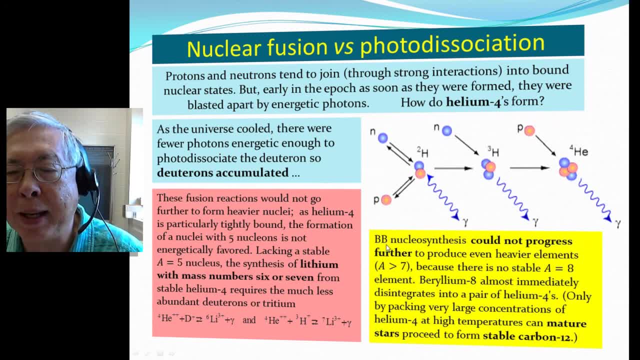 small Wow, so the big bang, Ecosys. it could not progress further. to bridges, even heavier, for example. so for for Maxim poets, you leăng n Labor de Van Long, and of above human beings, the Strogaard law scholars, improve the processes. very small score the conclusions of all of these changes. introduced myself to the founder of Ecosim, Valaya Abel, from Chicago State. so when these supporters were sitting together in Chicago, Europe, I must say so, the soy累ed product this project was Dzifism only so, of course, chestnut it was. 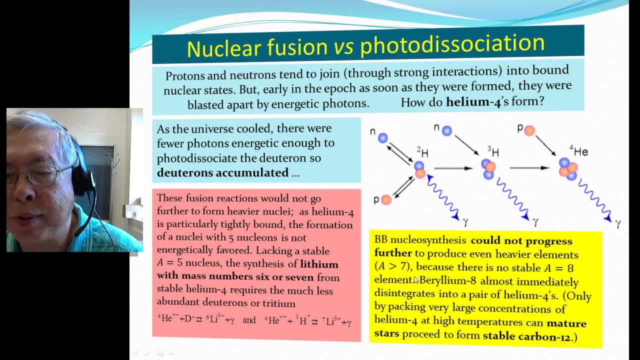 developed, for we don't kill to explore the再To be above human beings. seven, because there are no stable mass number eight elements, for example room eight, almost immediately disintegrate into a pair of helium force. so how the heaven? but only in the stars, when the packed very high concentration of 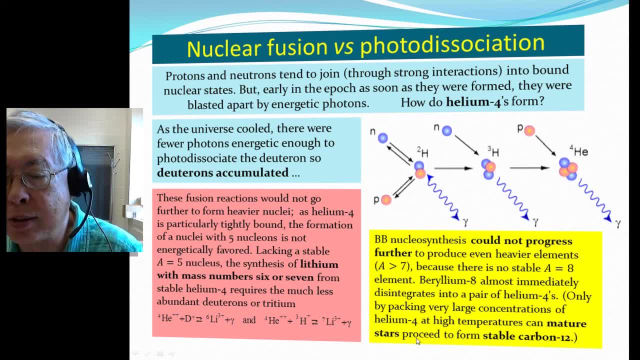 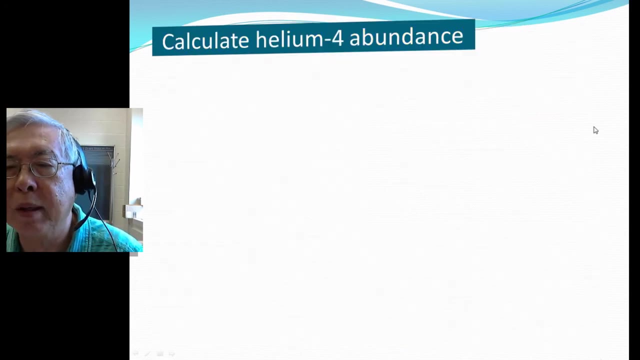 helium for it extra high temperature. can mature stars proceed to form stable carbon 12? so basically with all the heavy elements- carbon or those are pretty inside the stars, but here helium and deuterium lithium they will produce in the in a big band or in the early stage universe. so we can calculate the 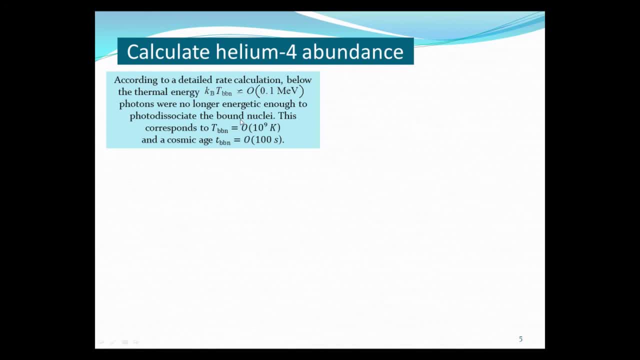 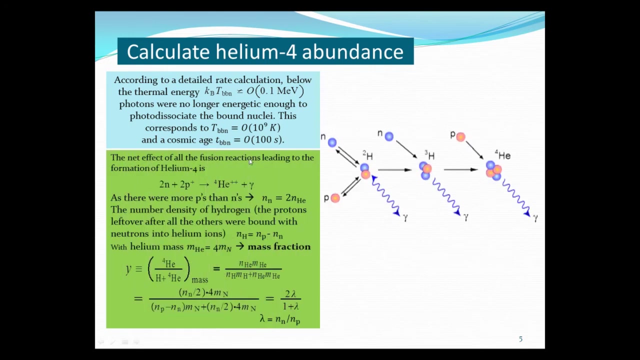 helium for abundance said. the gamma condition tells the big band you can stop at point 1 MeV and the photon no longer energetic enough to dissociate, bond. you guys. this correspond to the temperature brought- 10 billion, but about a billion Kelvin, and constant time about a hundred second. so then now we're talking about all this. 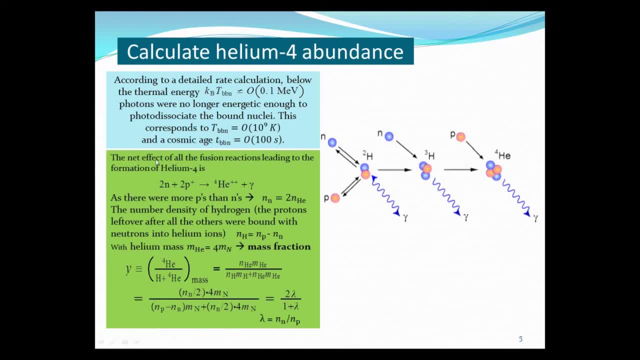 you can knows which planet-state power calls from Vari-C profit based on the gas, the at you give V of helium, because helium contains two neutrons, The number density of hydrogen, and which are the leftover from all the others. you know, it's all the protons that can be combined here. what's? 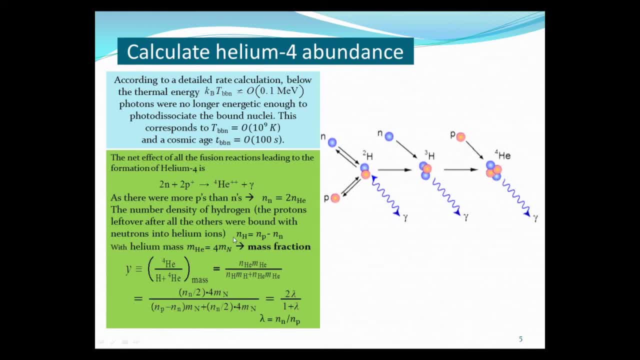 left over is the free protons, and so the hydrogen or hydrogen atom is equal to the number of proton minus the number of neutrons left over, become the hydrogen atom we see today. So now neutron proton basic mass is the same. we call it nuclear mass. and the helium had two. 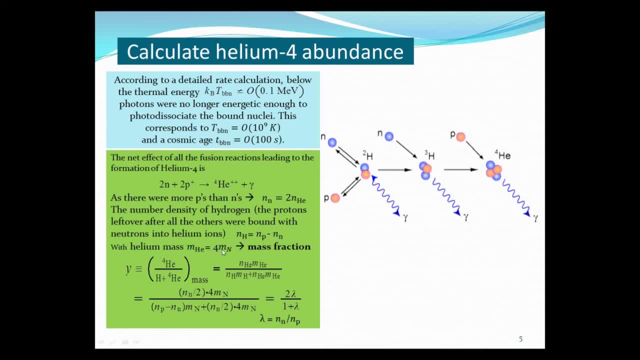 protons, two neutrons is four. mass is four times nuclear mass. so therefore the mass fraction- why remember we said about- is the mass of the helium divided by the sum of the proton or hydrogen plus helium-4 mass. okay, so therefore, the mass of the helium-4 is the number. 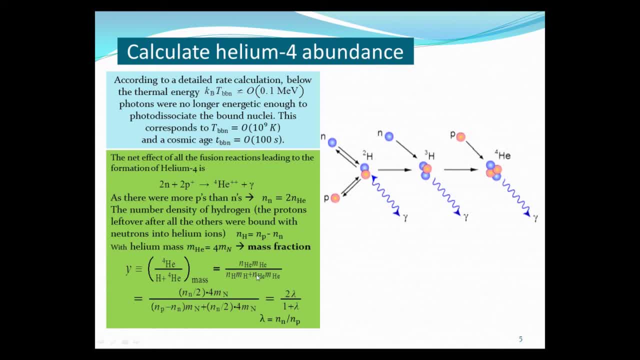 of helium-4 times the mass of helium and the individual helium atom. and same way the hydrogen is the number of hydrogen times the mass of the individual hydrogen. So n? h of n? e is- remember we talked about it's half- of neutron number and the number of hydrogen is proton minus neutron. so 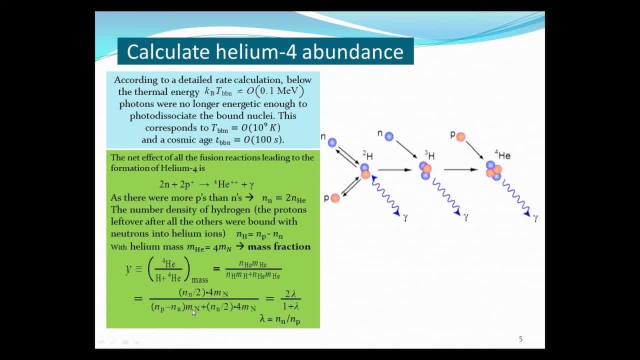 and the. the mass here is four times and of course hydrogen, it's just the one. proton is just so one nuclear mass. so now you can see, if I cancel all the nuclear mass factors and top is 2 divided by 4, divided by 2.2. 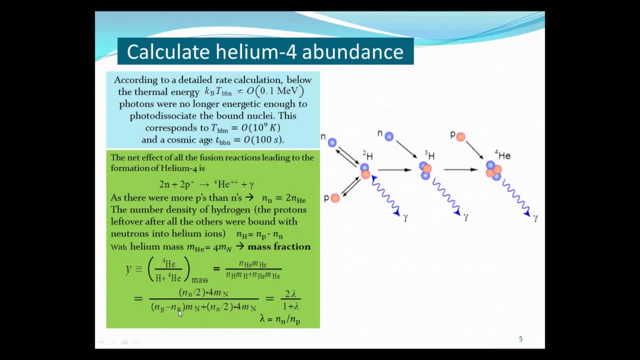 and then a whole thing divided by number of protons, so become N sub N, divided by N sub P, become lambda. same way, this is 1, this minus 1, so this is minus 1 is plus 2, so plus lambda. so therefore the mass fraction of helium is 2 lambda over 1 plus lambda. lambda is ratio of the neutral. 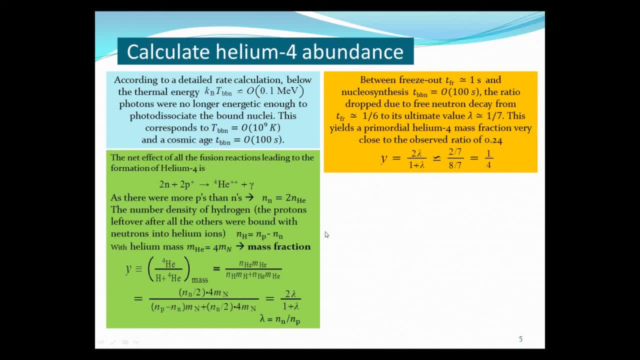 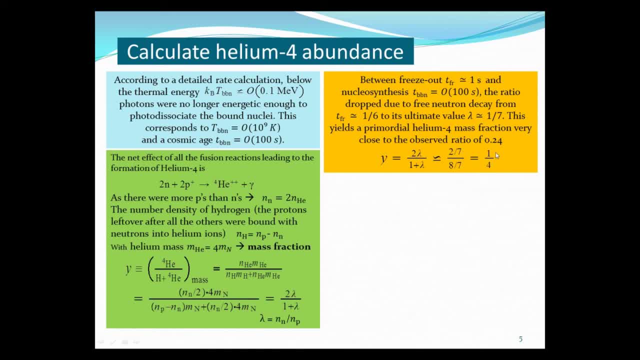 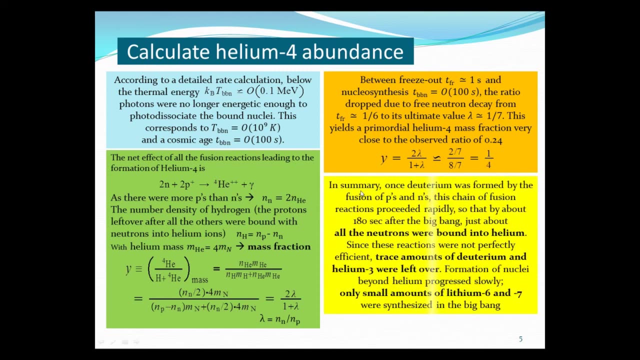 here, you plug in here, you plug in here, you plug in here. you got exactly point 2, 5. that's just very close to observe ratio and this, of course, is very crude calculation, more detailed calculation of both my equations and things, so be obviously more upset reaction rates. in summary, once the 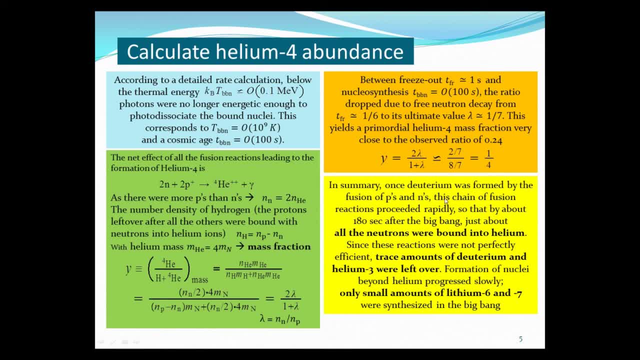 tutorial was formed by fusion proton, neutron. this chain fusion reaction preceded rapidly, so that's the by by, by beta Communications, by beta Communications, by beta Communications. since this reaction were not perfect, efficient, there are still traces about deuterium and helium-3 are left over. formation amputated young. healing progress slowly because only a small number of lithium, six and seven of synthesizing a big bank. 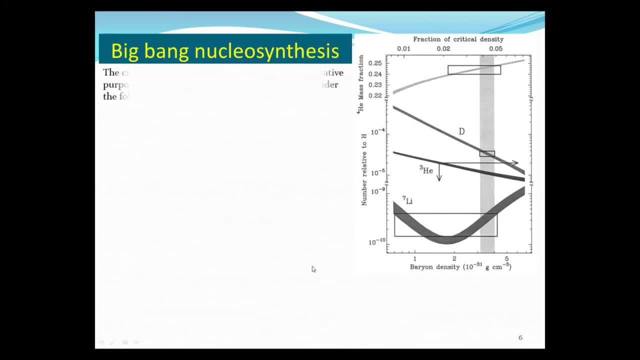 egyo in here. I'll explain this diagram later. So the crew calculation presented here is for illustrative purpose only. But realistic calculation would consider, for example, the fact the standard model assumes free flavor of light neutrinos, electron neutrinos, muon neutrinos, tau neutrinos. 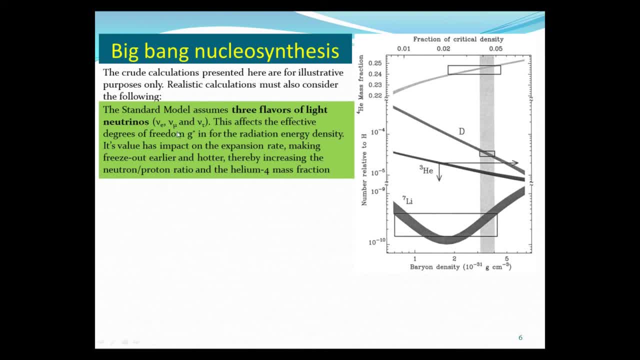 This affects the effective degree of freedom For the countine speed degree of freedom in the radiation energy density. it has an impact on the expansion rate, making it freeze out earlier, harder, thereby increasing the neutron proton ratio and affects the helium fraction. 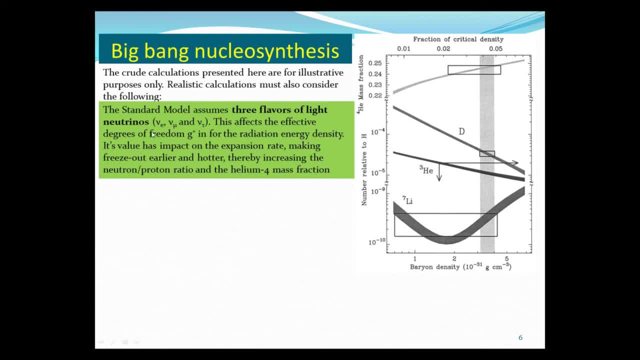 So the fact you had to take the fact that there are three neutrinos, In fact the fact, the first evidence that only three neutrinos are free, Three light neutrinos came from cosmology, not came from particle physics experiments. Also, this light element abundance turns out depends on the barrier of mass density. 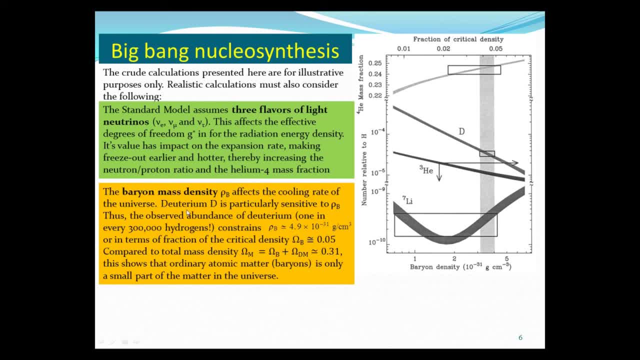 Because it affects the cooling rate of the universe. In particular, deuterium is particularly sensitive to the barrier of mass density. This observed abundance of deuterium- one in every 300,000 hydrogens- constrains what this value would be. 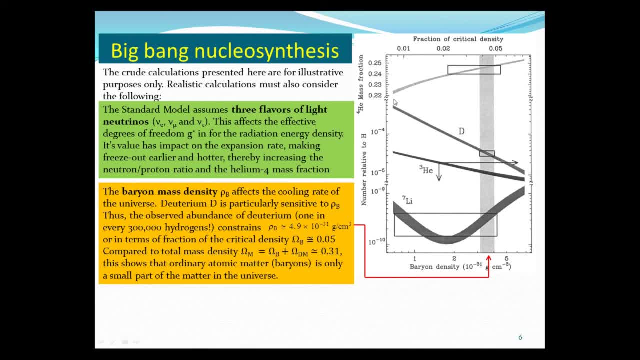 Here is a plot of a theoretical calculation of helium. Here is the 525.. But it turns out this fraction depends on the barrier of mass density. This fraction depends on the barrier of mass density. This fraction depends on the barrier of mass density. 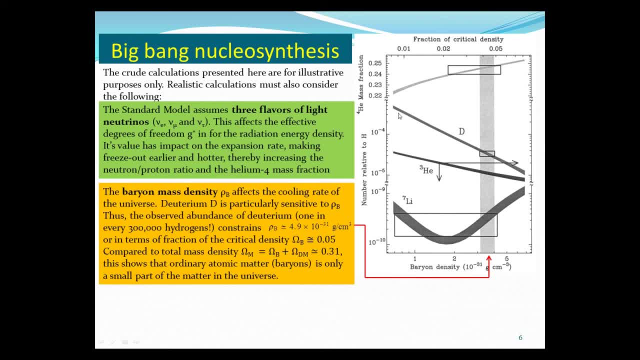 So helium dependence is not too strong, but it depends on it. The most strong dependency is deuterium. It really depends on the barrier of the barrier of mass density, And helium-3 also depends on it, but again not too strong. Lithium depends more strongly. 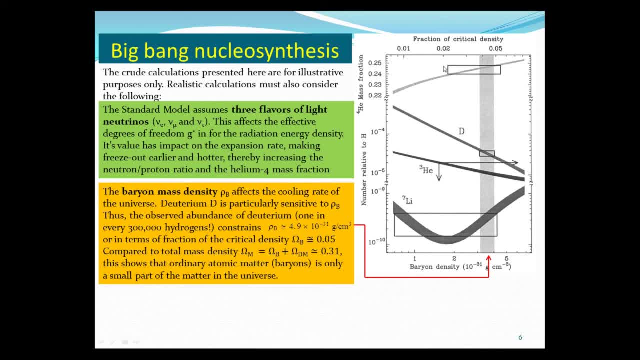 Now, these curves are the theoretical curves, curves and the vertical width, vertical height, if you want, is the observation of uncertainty, And the term is very well defined: it's very narrow. So therefore, this box indicates the value of barrier mass density and those compatible. 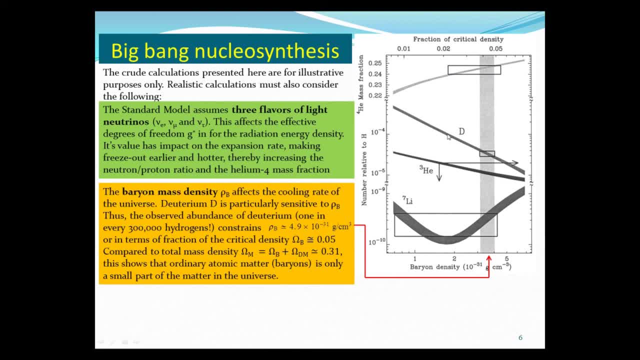 theoretical predictions: Same because the term depends on. it's a very strong dependence and it's very well measured. so it fixed the barrier mass very well to a narrow range And here it's not very good. but lithium is also not very good. 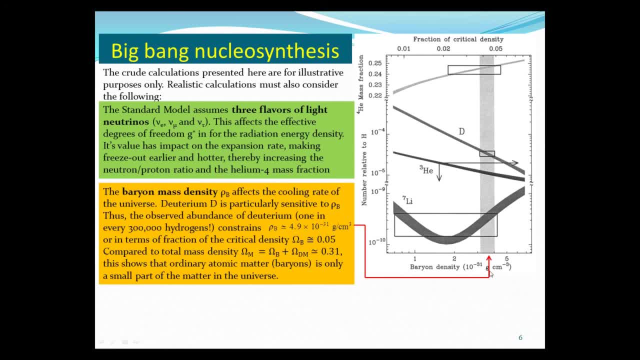 So mainly, it determines the value of the barrier mass density to be 4.19 to minus 31 grams per second. Okay, Now the same way in terms of the omega. so the density parameter is about 5%, or in fact, by the way, this graph is kind of old, about 10 years, more than 10 years old. 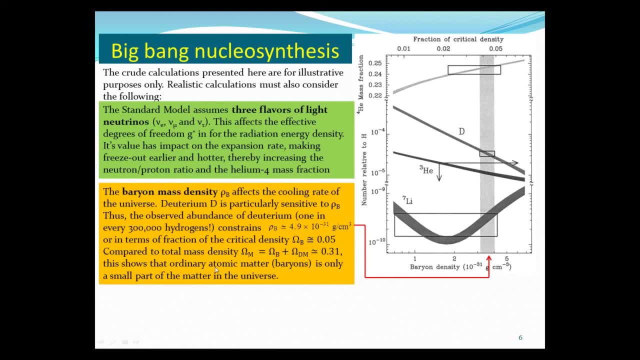 So now the value drifted a little bit more towards 5%. Now compare the total mass density. remember we said Okay, But this is 5.1, and this shows that the ordinary atomic mass, the barrier, is only a small part. 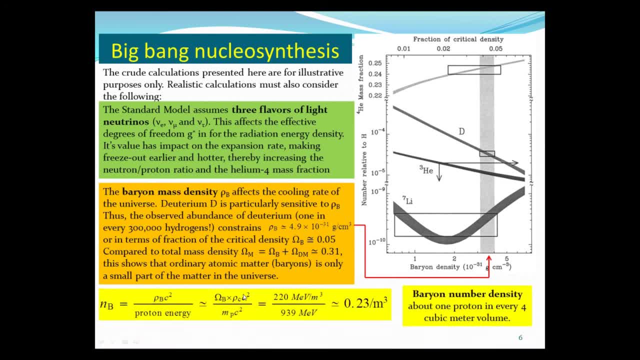 of the matter in the universe. Now, once you know the from here, notice the barrier mass density. you can divide it by the or proton energy. So the barrier mass density is the parameter omega b times critical density. Okay, So the barrier mass density is the parameter omega b times critical density. 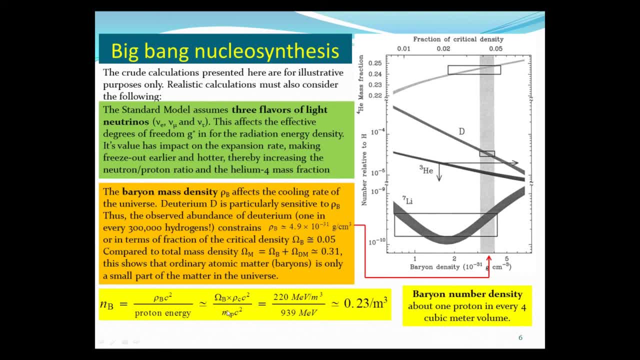 Okay, protein is based on rest energy, so that's 939 MeV and this 0.5% times the critical density is about 220 MeV over per cubic meter, so you get 0.25 for cubic meter. So therefore the baron number density is about one proton in every four cubic meter volume. 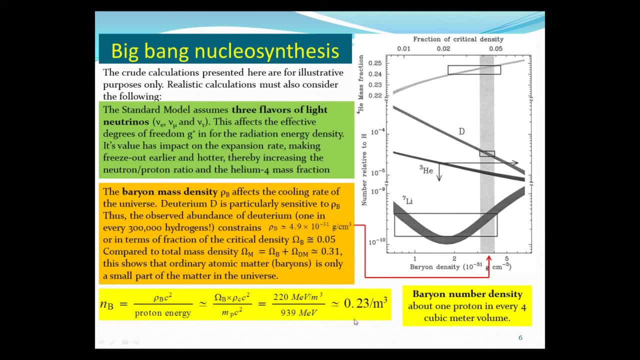 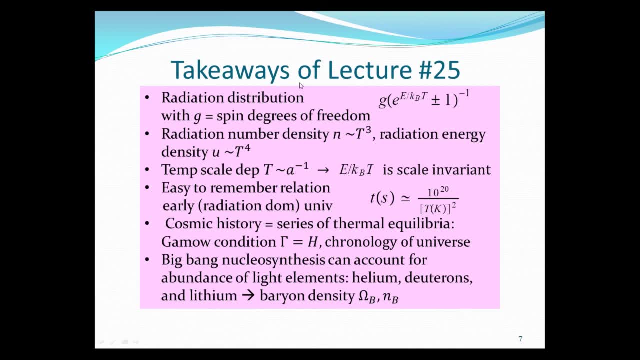 Again, it's an extremely small number. Okay, we'll talk about the lesson we learned in lecture 25.. We said the radiation distribution is the standard which you're learning in physical physics. is the g is the spin degree of freedom divided by a factor: e to the e to the kt. 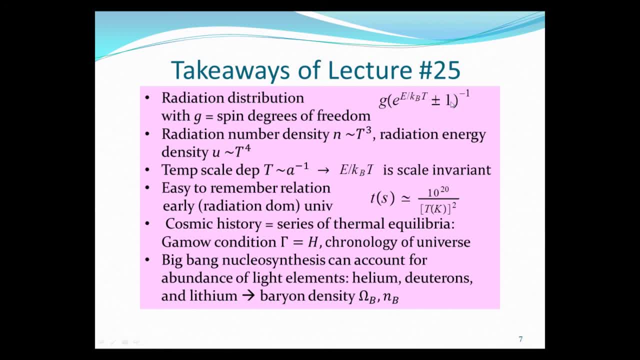 plus one for fermions, minus one for both. So you get your fu and you have your mu, And then you have a distance n, which is the distance between two photons. one photon and the radiation number density is. if you integrate that this is the n, we get the temperature. 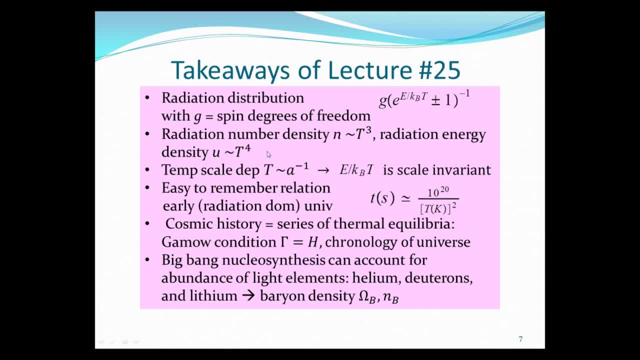 to the cube. and same way. if you sum up the total radiation energy, the energy density is proportional to the fourth power temperature, that's over A, and so therefore E scales up one over A, KT scales one over A. so therefore the combination E over T is scale invariant. so this distribution do not. 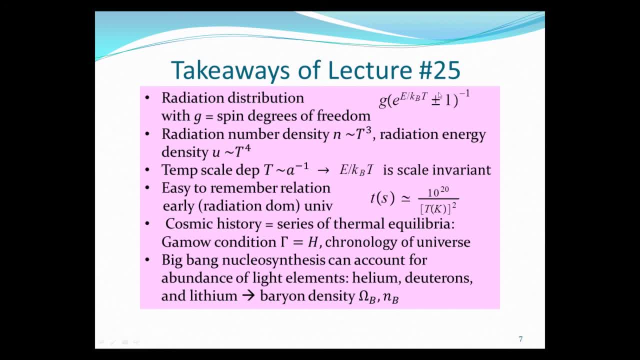 change, even though the temperature getting cooler, a lower, lower, but the distribution still same. and easy to remember the fact. you can from the temperature you can figure out what constant time was the radiation was this system? so the cost of a history is composed of Sears, thermal equilibria and 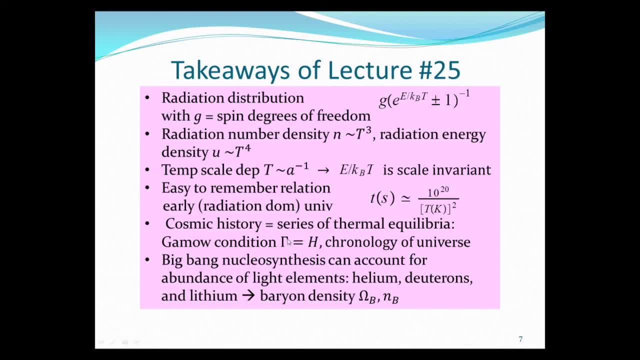 the transition time is determined by the reaction rate versus expansion rate, and from this we can form a chronology of the universe and the Big Bang Euclid thesis can come for abundance, light elements, helium, deuterium, lithium, and from this we can deduce the baryon density. 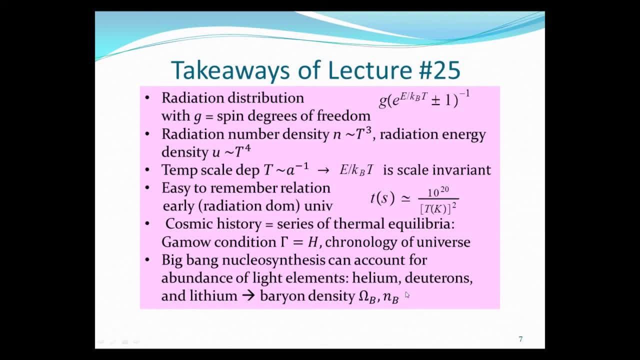 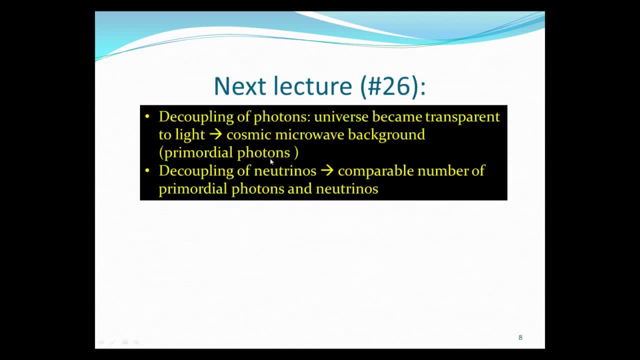 you omega-b or number density, number of baryon per unit volume. for next lecture, we're going to talk about the copying photons when the universe become transparent to light and David. so these are the primordial light of water photon, which is the constant microwave background we have detect today at the 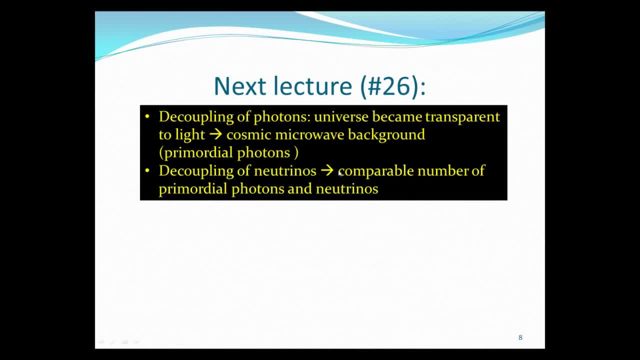 cup also. similarly, there's the copy of neutrinos. so it turns out you can calculate the light of neutrinos and you can calculate the light of neutrinos now, if I have any of these electrons present and we work with a computer and they're working, now we can calculate the light of the neutrinos. 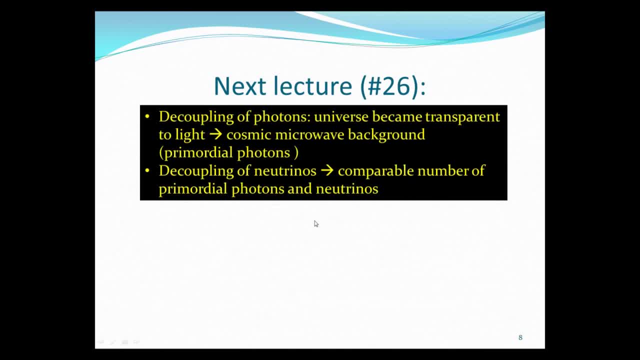 these electrons are now interesting. the light of neutrinos is the number of electrons present in the universe will be the number of electrons present in the universe.